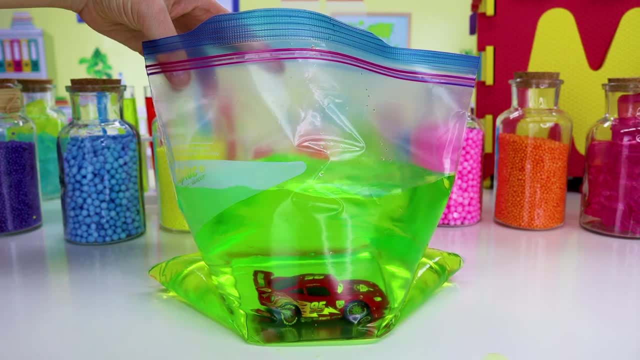 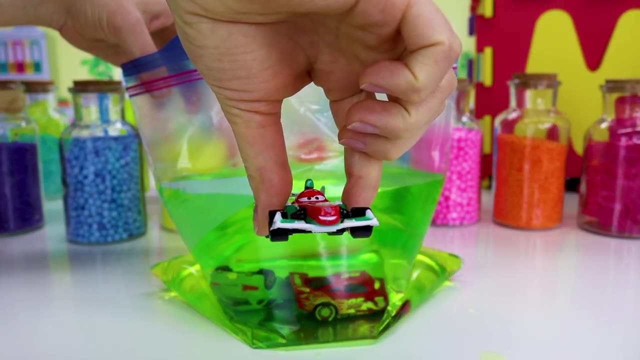 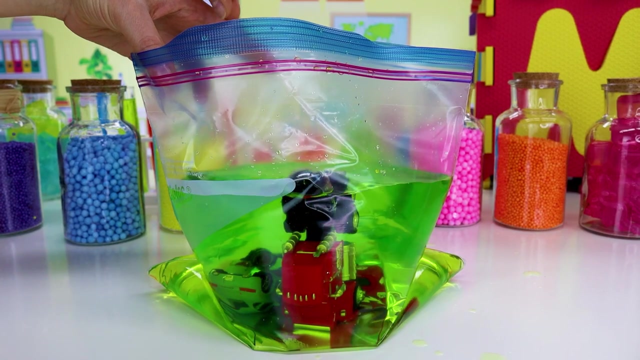 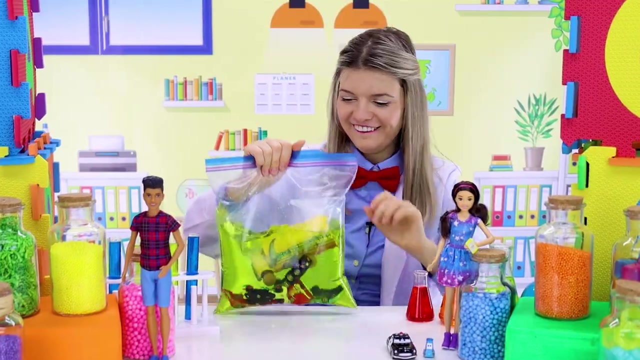 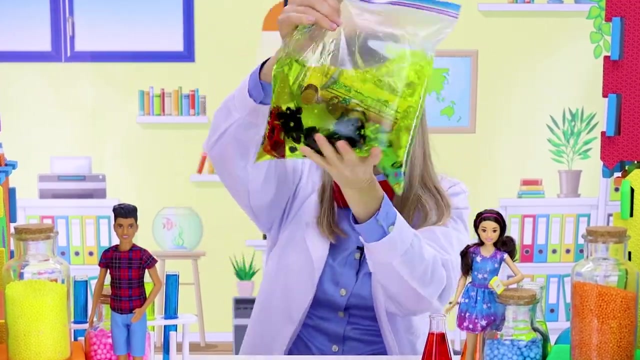 Bye bye McQueen, Bye bye Sally, Bye bye Francesco, Bye bye bak, Bye bye Miss Fri-ter. This is getting really heavy. I think that's enough. Dance, dance, dance, dance, meet the guys. 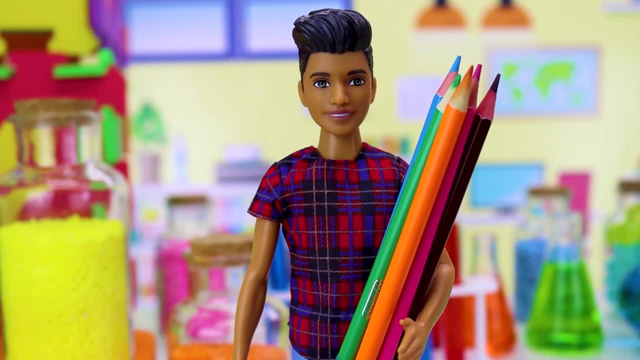 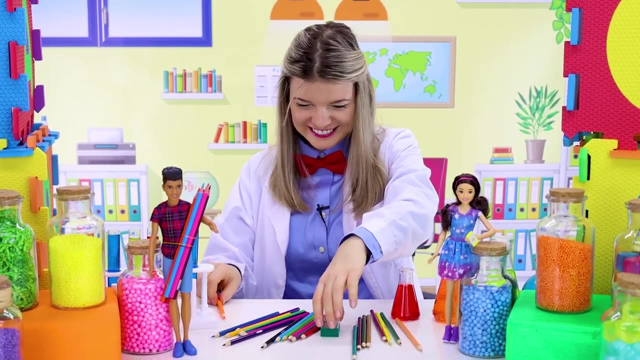 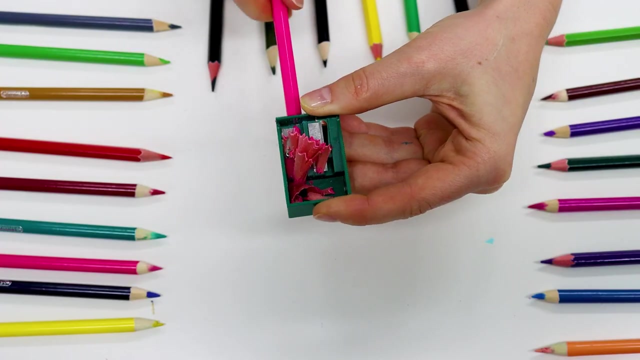 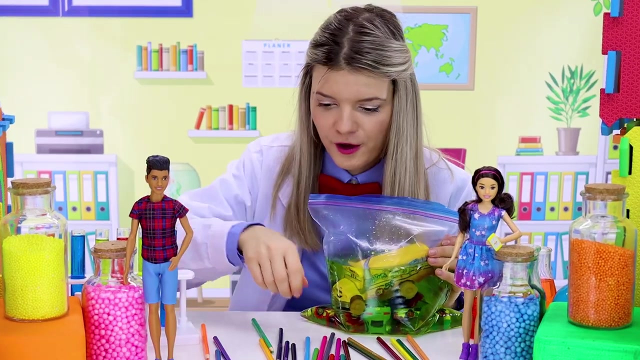 Woo, woo, woo, woo, Woo woo. Hey, Deedee, we need to sharpen our pencils. Alright, and don't forget to ask an adult for help. Let's sharpen, Okay, our pencils are ready. Now we'll take a pencil and put it through the bag of water. 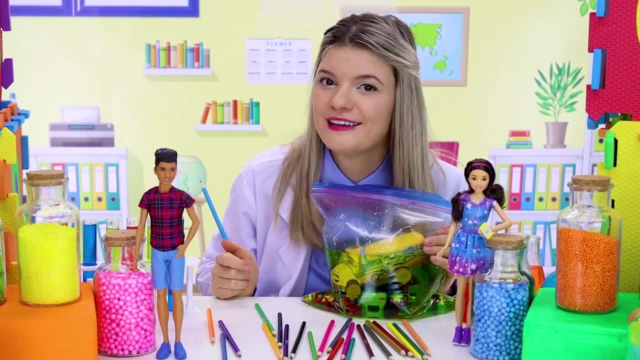 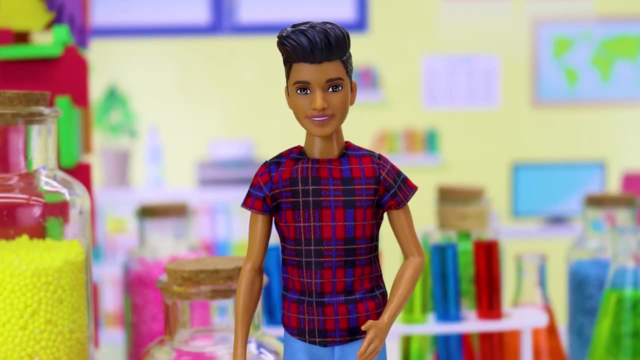 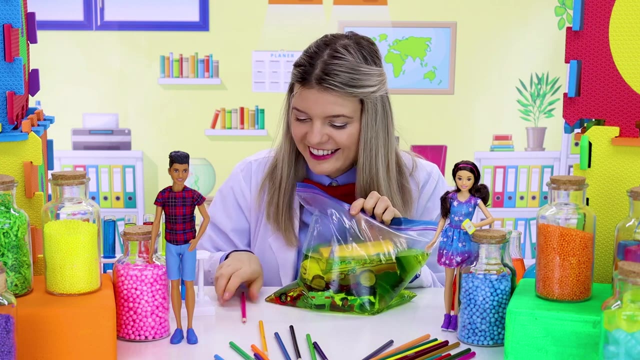 What do you think will happen? Do you think the bag is gonna leak, or do you guys think it's not gonna leak? Huh, Oh, it's definitely gonna leak. Um, I really don't know. Okay, let's test it and see. 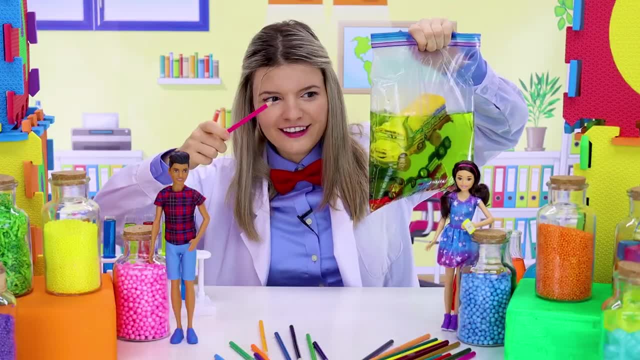 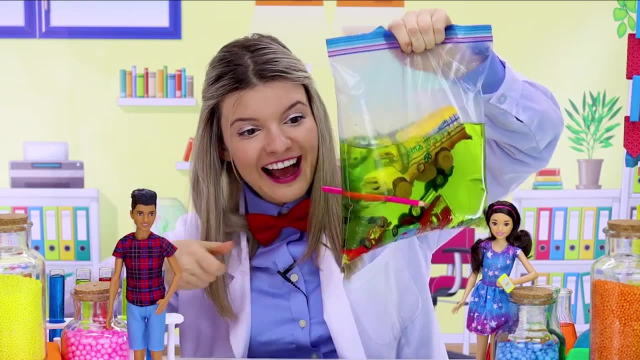 Ha, Dum-da-dum, Are you ready? Woo, Oh, did it leak? Oh, look at that, It's out on both sides. Oh, look at that, It's out on both sides. Oh, look at that, It's out on both sides. 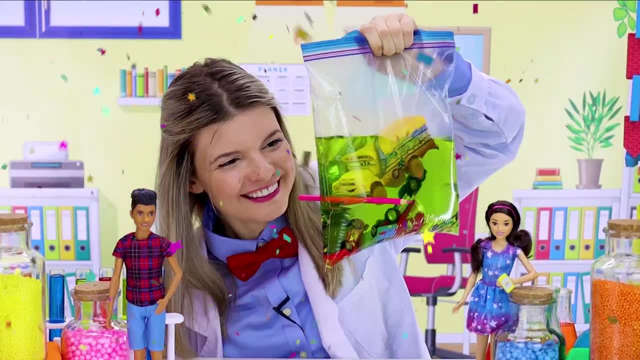 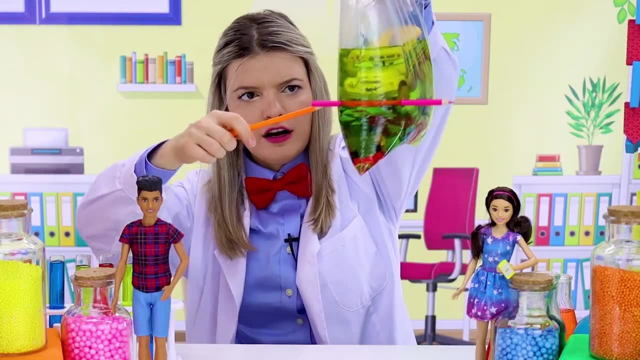 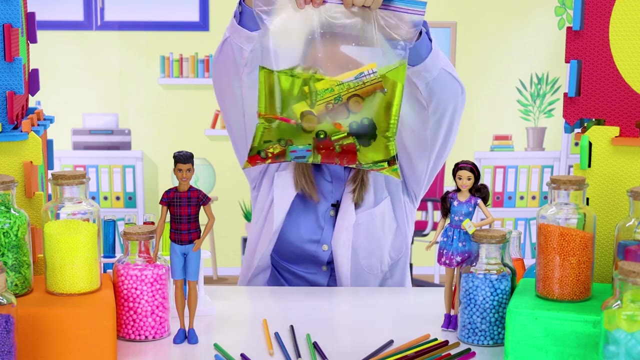 And it's not leaking. Woo-hoo, That's so cool, Let's put some more pencils. Sounds good to me. We'll take orange. Ha Dum-dum-dum, One And two. It's out and not leaking. 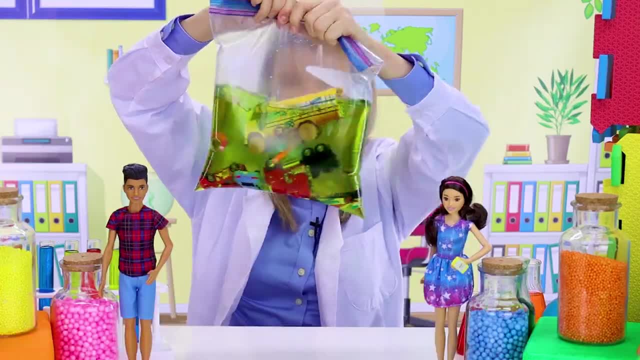 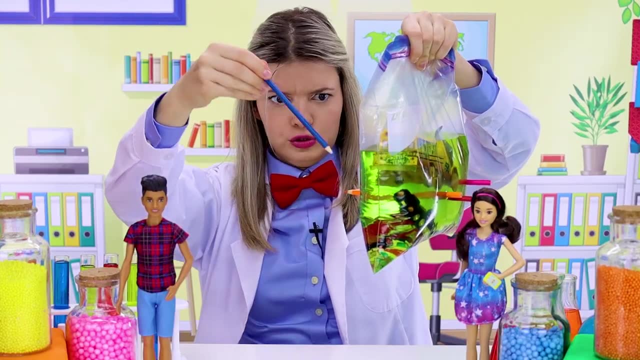 Woo, Sorry, Barbie, Come back. Woo, Okay, got them. What if we do them on an angle? Let's try: Ready, Ready, Choo-choo-choo-choo-choo, Boink, Boink. 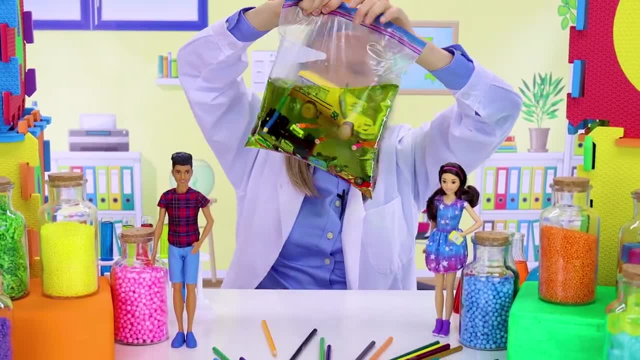 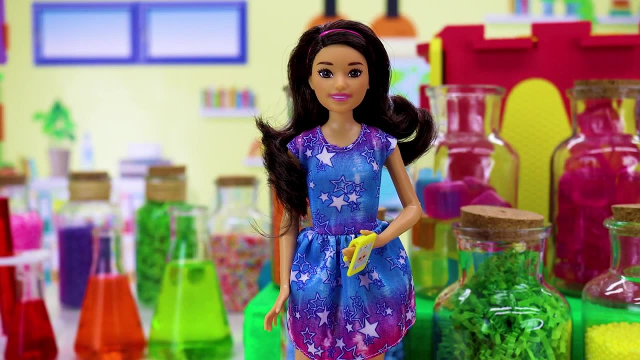 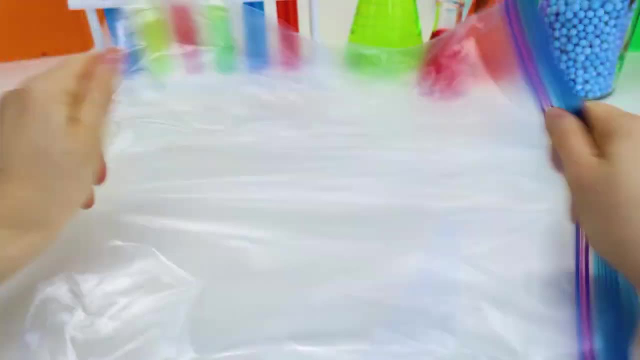 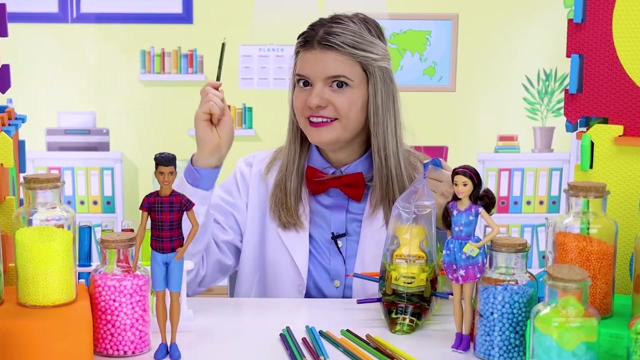 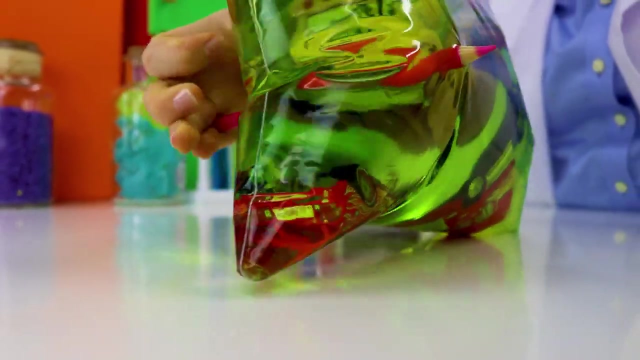 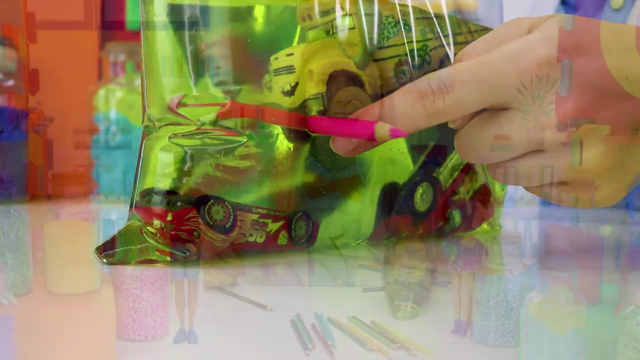 Ah, It's working, No leaks. But I don't understand Why doesn't it leak? That's a great question. The bag is made out of this stretchy and flexible material called polymer, And when we put a pencil through it, it seals around the pencil and doesn't let the water leak. Pretty cool, huh. 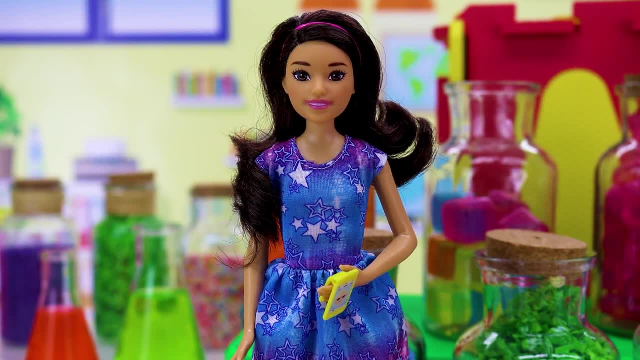 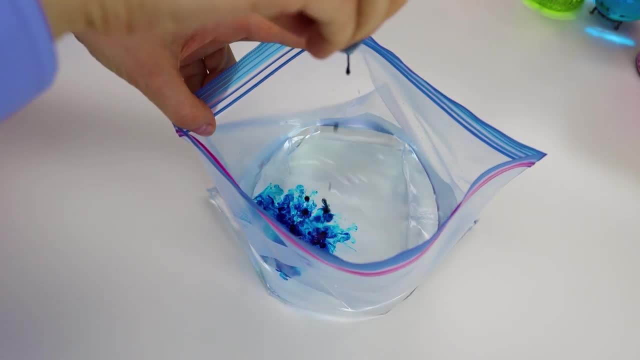 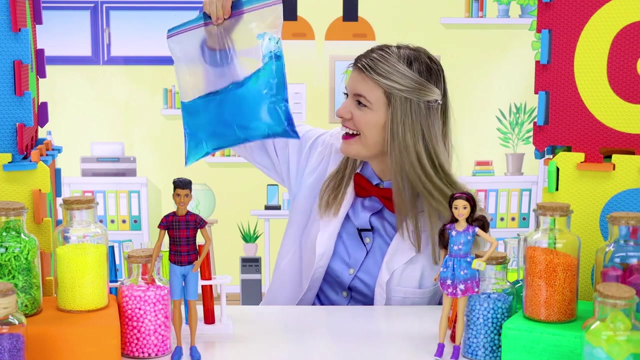 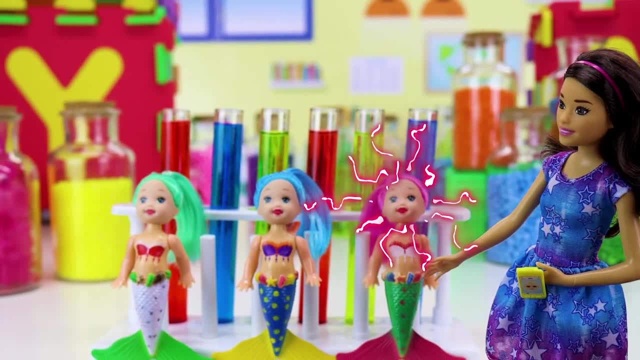 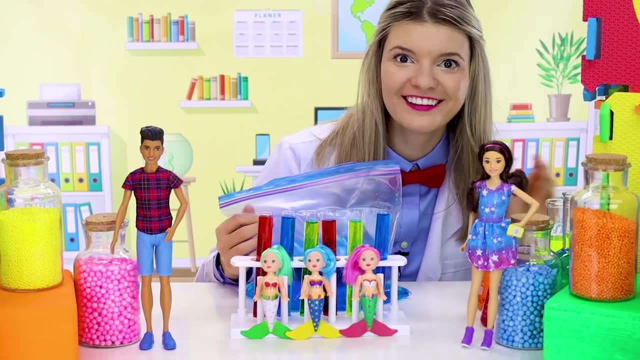 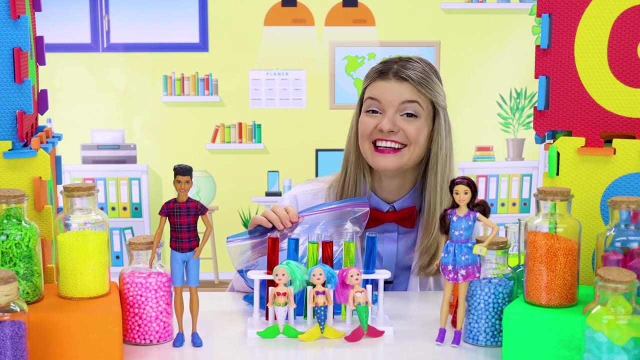 I want to put my mermaid friends Anna, Banna and Banana. They're the best. Wow, Hello mermaids, Ready to go for a swim-swim? Yeah, Okay, let's go Swim, swim, Anna. 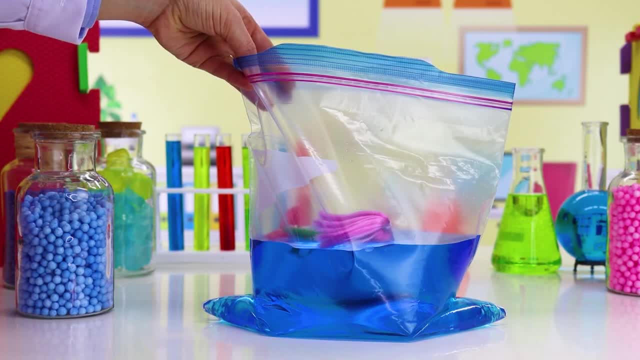 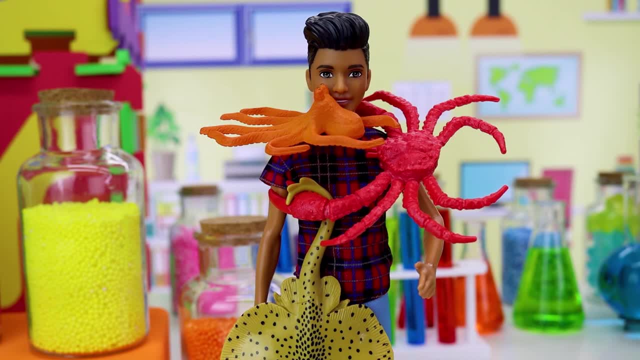 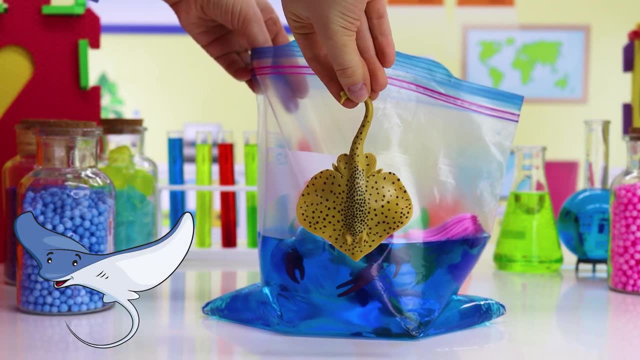 Swim, swim, Banna Diddy, let's add some sea animals. Bye-bye crabby crab. Bye-bye crabby crab. Goodbye Mr Stingray. Goodbye Mr Stingray, Adios octopus. 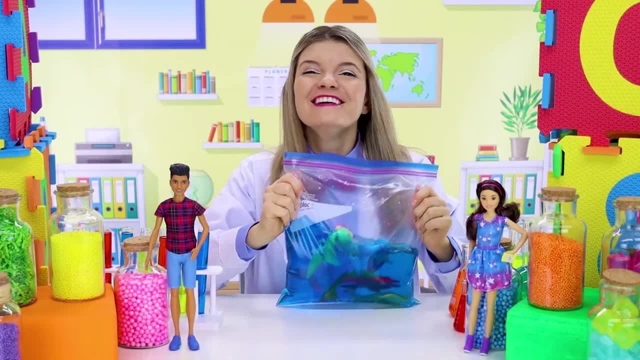 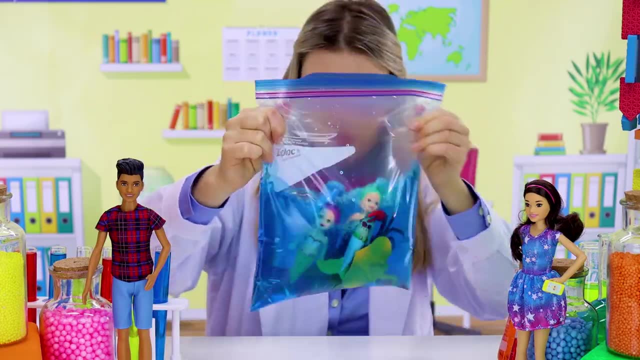 Adios octopus. Woohoo, We got mermaids in the ocean. Mermaids in the ocean, Doo-doo-doo-doo-doo-doo, Mermaids in the ocean, Mermaids in the ocean, So fun.